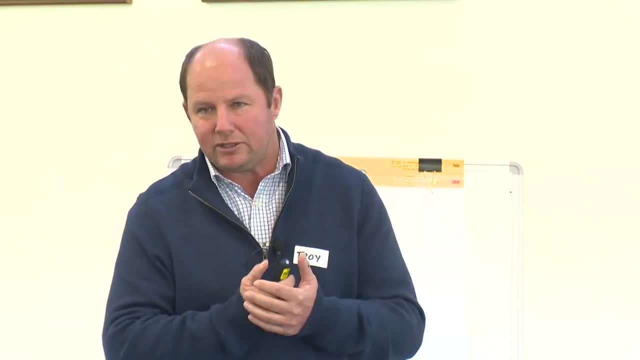 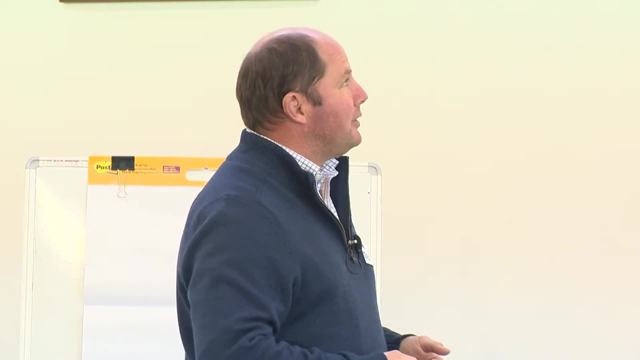 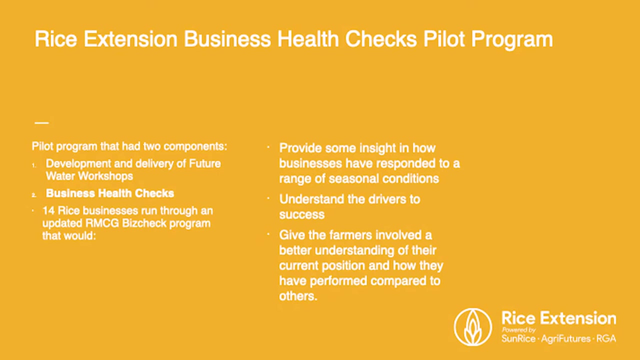 that successful. we did get some assistance from the Rural Financial Counselling Service to get a few more on board, but what we did end up with is about 14 businesses. So yeah, and we thought we'll put this program together. so it was two parts: develop and deliver some future water workshops, which I'm pretty sure. 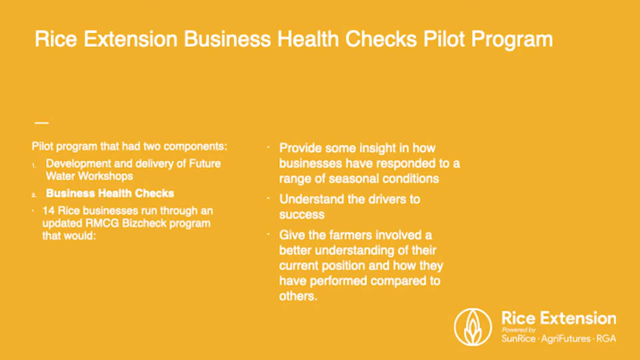 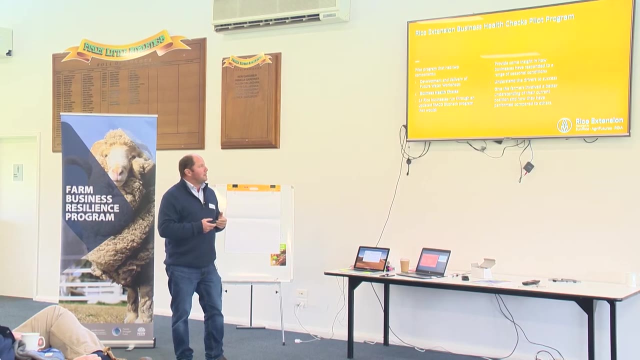 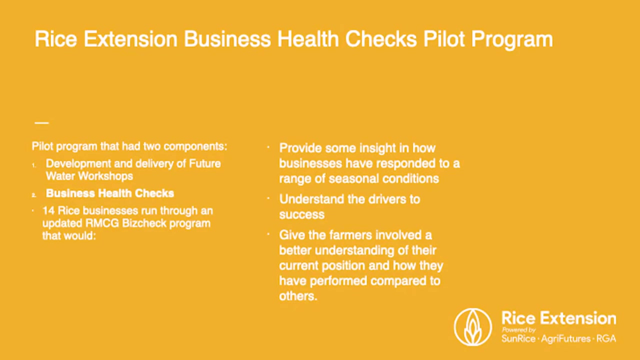 Rob will touch on a lot of that work that we discussed in their workshops. and the second part was these business health checks, as I said so. so the aim was to provide insight into how they, those businesses, responded to different allocations, different seasons, understand the drivers the success and give the 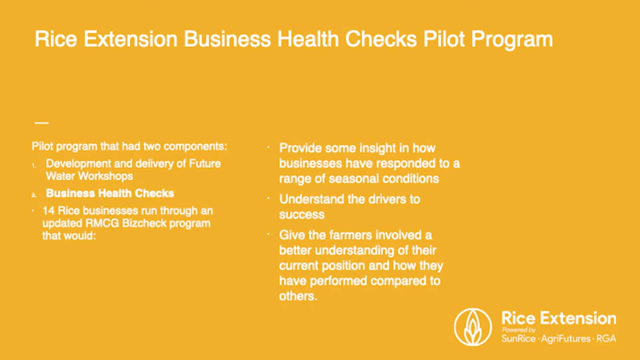 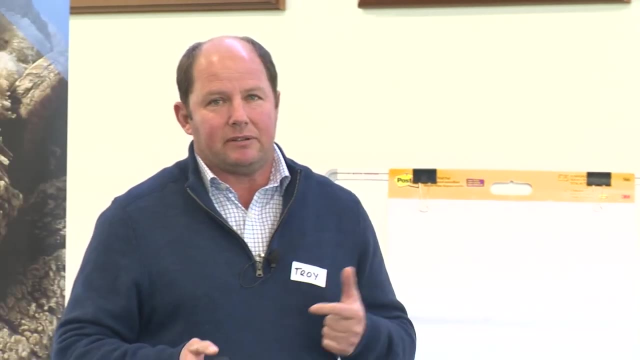 farmers involved a better understanding their current position and how they stacked up against their peers or other people within the Murray Valley. so first step was we had to look at where are we now. so we had to collect some information. we went from the 16-17 season, which was obviously very wet. we 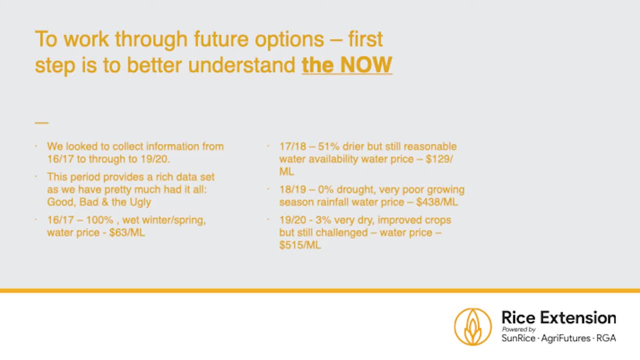 had 100% allocation that year. the average temporary water price was 63 megaliters of 63 dollars a megalitre. all these averages were the average of the MIL water exchange, so that's was our source of data for that. so that was the first step, and then the second step was to look at the 17-18, which was a dry year, 18-19, which obviously had 0% allocation, and 19-20, we had that late 3% allocation. I think we've got in May or something like that. so so, as you can see that from the data we collected, we had good seasons average. 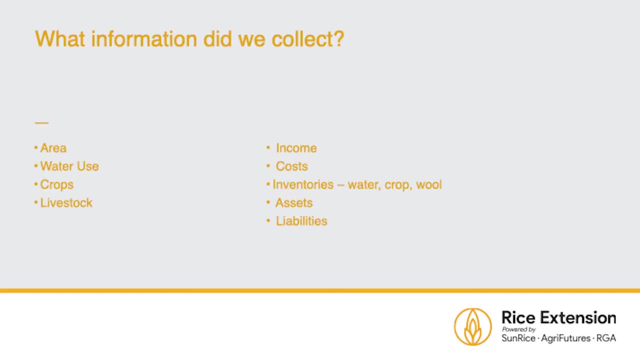 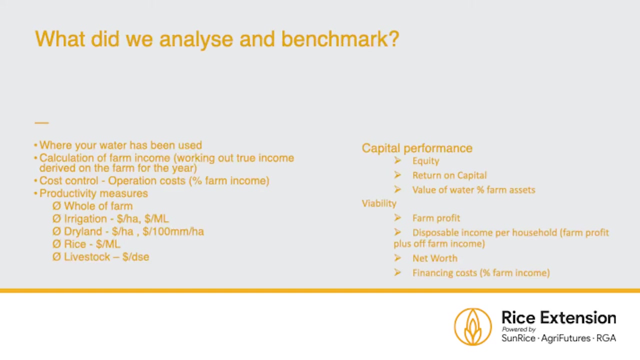 seasons and very poor seasons. so that was the data we collected. what did we collect? area, simple things about area: water use, crops grown, lifestyle and other things, income, our costs, our inventories that we held over or from season to season, how they change assets and liabilities. so briefly, what did we analyze? where the 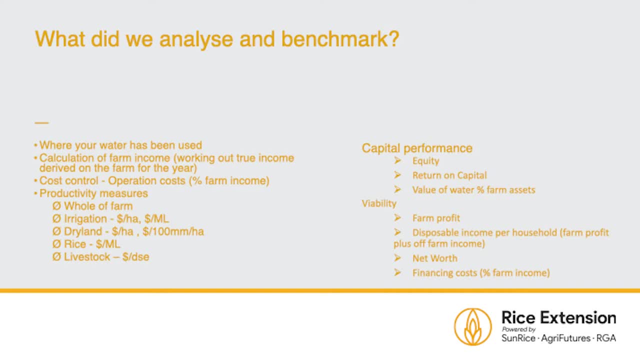 water had been used. calculation of farm income and this is working out the true income derived from that farm from that year. so not, so it was the match, all the costs and income with one financial year. so we, particularly of rice, as we know, we get payments in the second and third year. 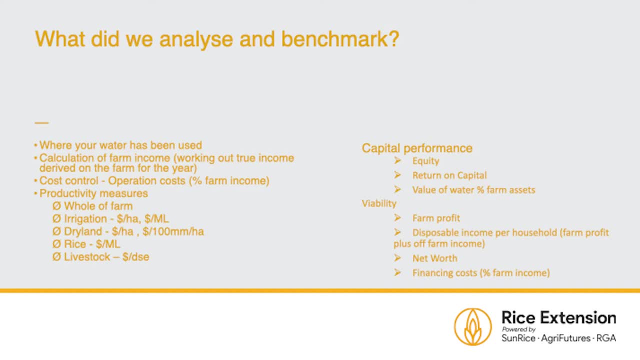 so it's a pull them into one year to see whether that year was profitable or not. so it took a bit of doing. the productivity measures were whole of farm irrigation- dollars per hectare and dollars per meg, etc, etc. and then we went to capital performance and viability. so we did a few yeah, measurements and 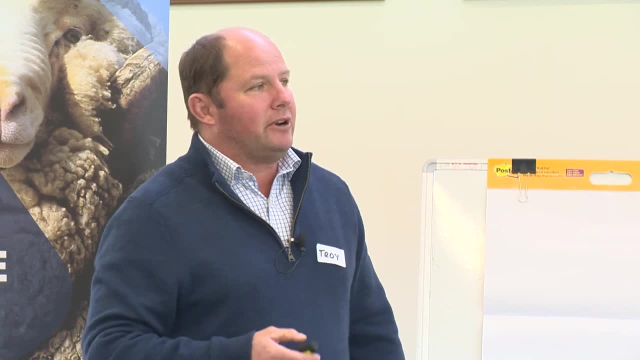 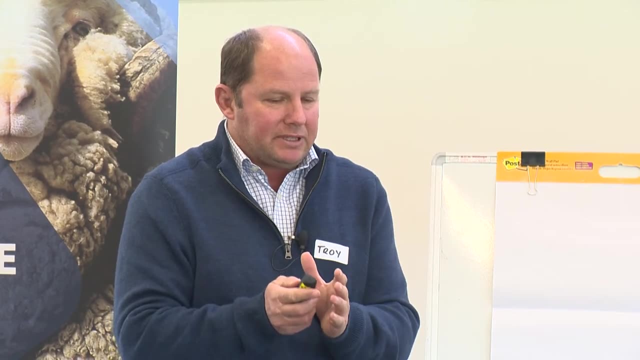 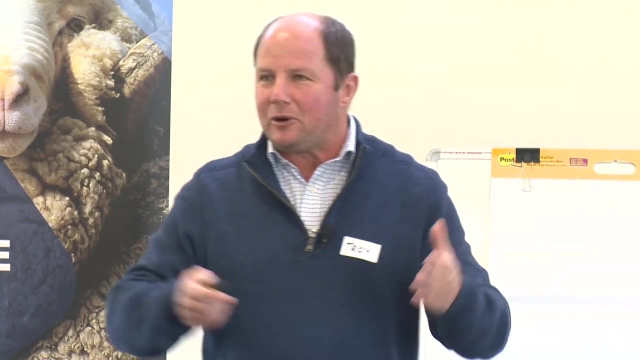 benchmarking. so of the 14 enterprises that were involved, not all of them did the whole four years, because we did do this in, not in 2021. so to look back at historical records, we all aren't good at keeping records of our farm management practices, so it was a bit difficult for. 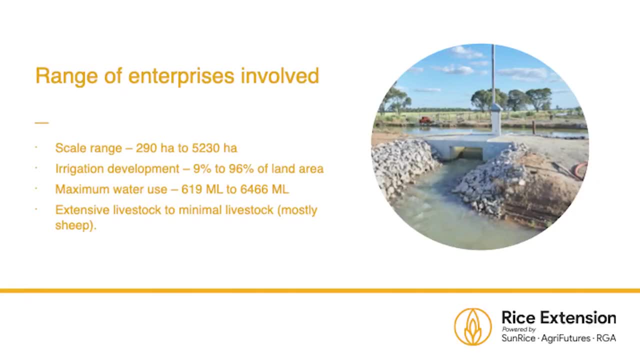 some, so not everyone, did the four years. but so the range of farms was from 290 hectares to 5,230 hectares. so we had a good range, good spread of farms. of them, farms, the irrigation development of the irrigation development, of the irrigation development was from 9% to 96% of the land area and the maximum water use in a 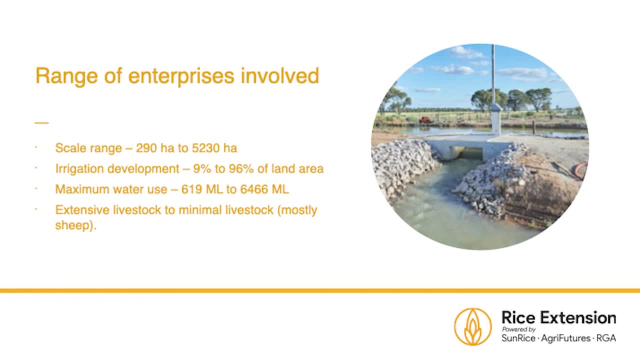 good year of these farms was 619 megs to 6466, so a real. just to try and show there was a real breadth of some of participants we had and that's what we really wanted. we really wanted to look at each end of the scale. so and yeah, 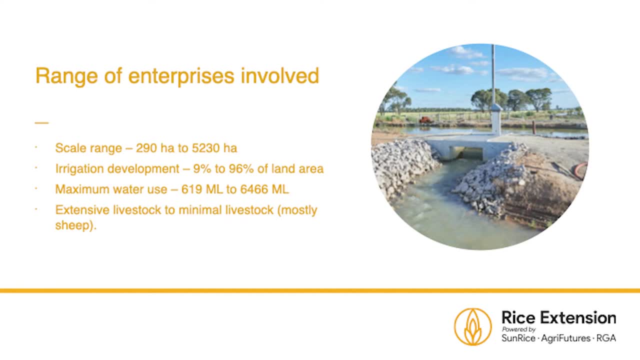 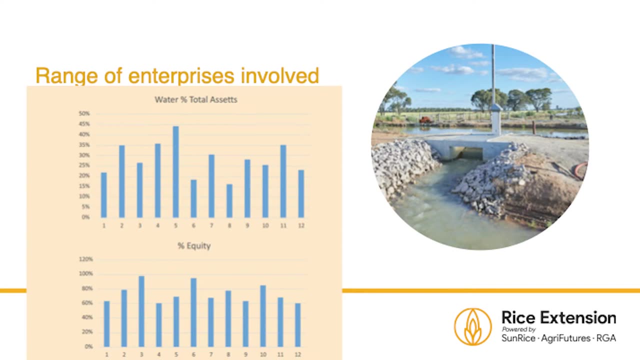 obviously extensive livestock to minimal and mostly of the livestock had sheep. so just a little bit more insight into the farms. you can see the water percent of total assets range from just a little bit under 45% down to 16%. so that's that top graph. so they're the farms, the numbers of 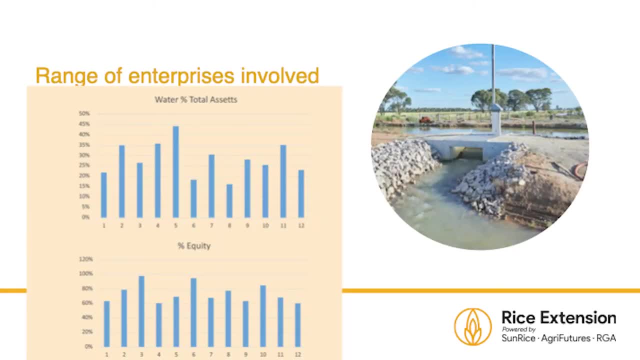 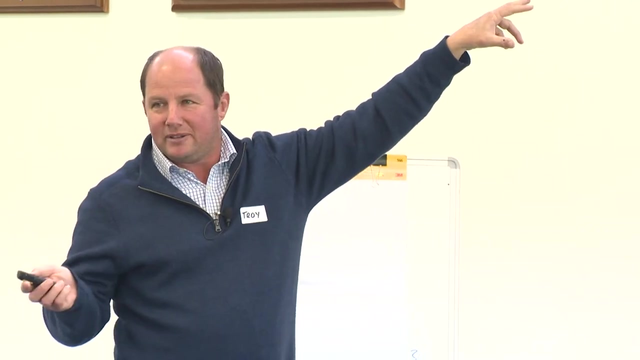 represent a farm. so yeah, so if someone had like the 45%, if he had 2 million in total assets, he had about nine hundred thousand dollars worth of water. maybe that would be the means of bombs up using that, which would get up that portfolio. so so there was a fair spread and it just indicates what we all now in. 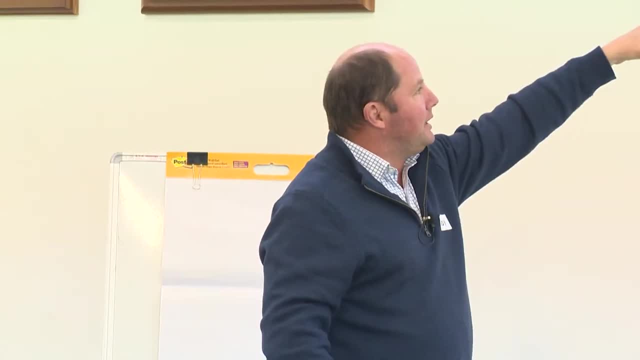 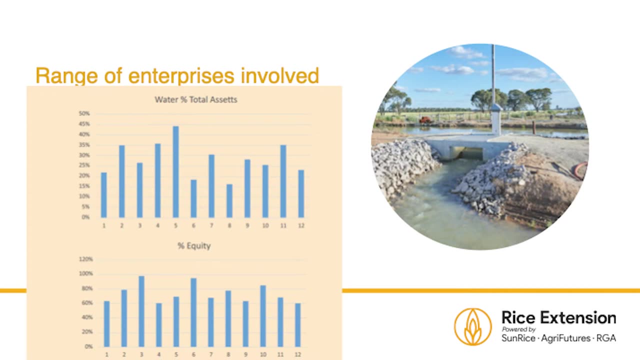 Marie Gianna, not every farms the same, so some have lots of water, some have less the equity. so just yeah, there's also a couple just a touch under 100% and then down to as little as the 60% equity. so we had a good range there. 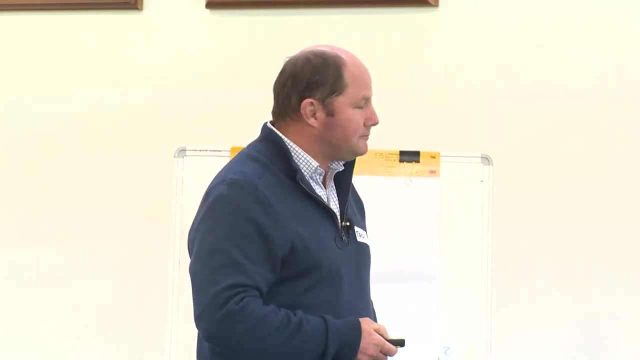 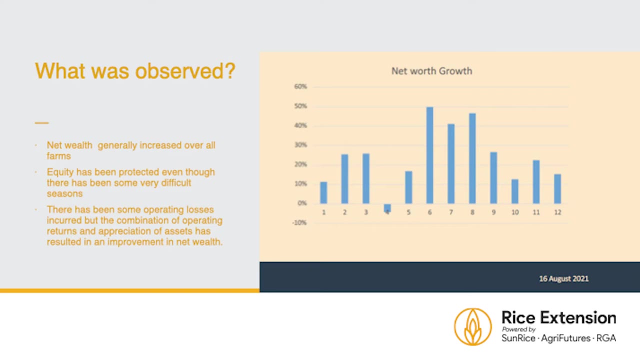 you know, obviously there is farms out there with less equity, but we didn't, but it's still, once again, a pretty good range. so what do we observe from all this? uh, generally net worth, um, we had growth in most farms, just about all farms. why is that? over that period- so we're thinking from 1617 to 2021- what's happened? 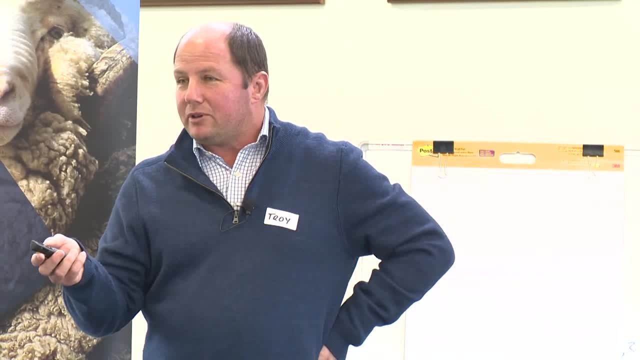 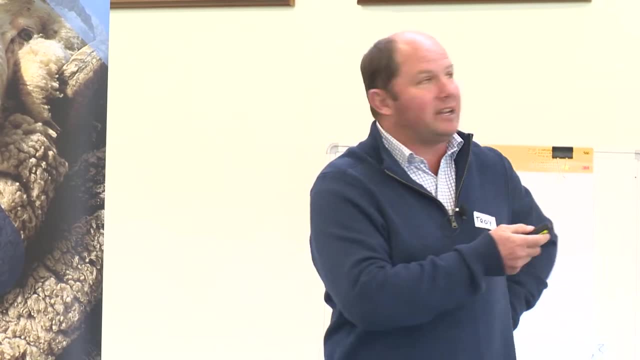 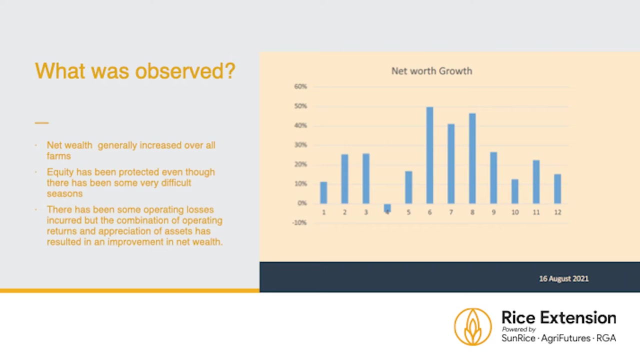 water a little bit, yeah, but what's really going up? what's helped us? land prices and livestock prices have really skyrocketed since then, so that really helped everyone. so, as you can see, some you know someone had 50 net worth growth over them four years. so amazing, which we, i'm pretty sure you. 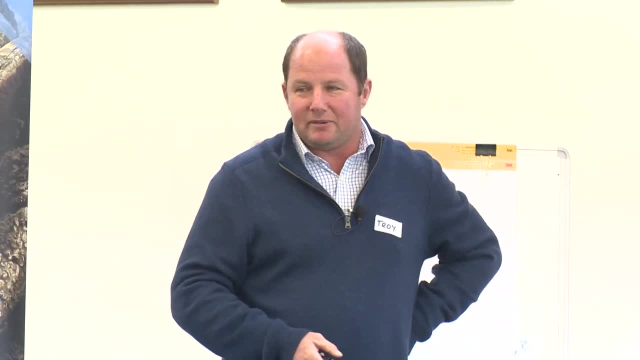 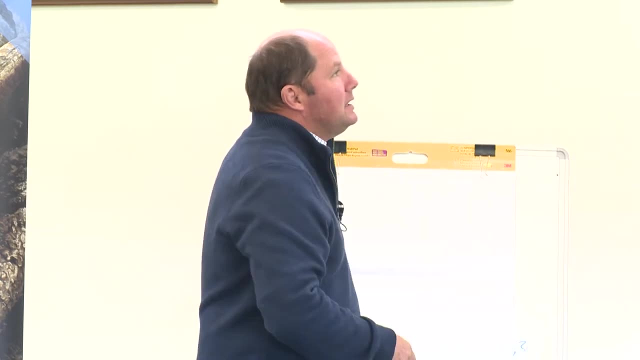 know land was selling for eighteen hundred dollars an acre around here and we thought that was expensive. now it's selling for 3400. you know it's just gone up that quick, so that's reflected in those results. uh, equity has been protected even though we had some difficult seasons. so you remember in there in them four years, we had two years of zero allocation, so it was pretty protected and that obviously was operating losses incurred. but the combat combination of our appreciation and returns resulted in improvement of net wealth. rob, jump in if, uh, if i've missed anything or you got. 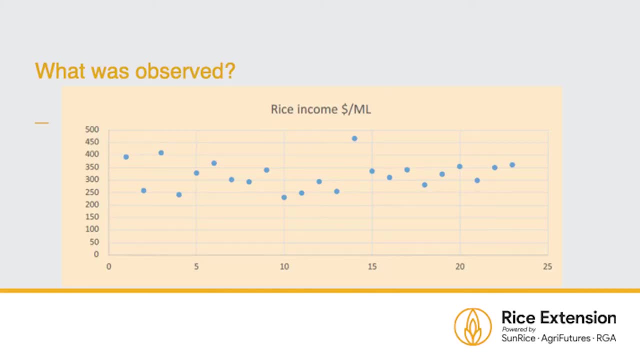 something to add. um, so also what was observed? there was a big range of income per megalitre from rice crops. so we can see there's a, you know it ranges from 475. so this is purely income: 475 per meg down to 250 dollars, and that's important and you'll see a little bit later. so yeah, they're. 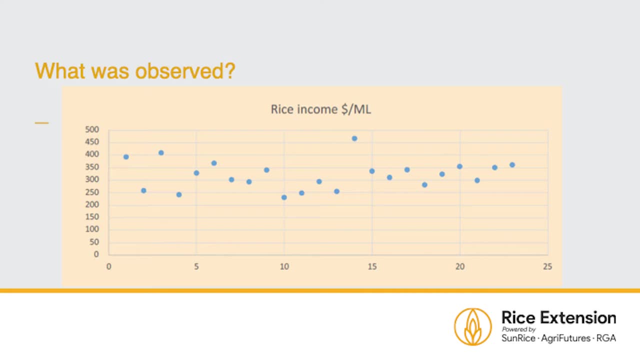 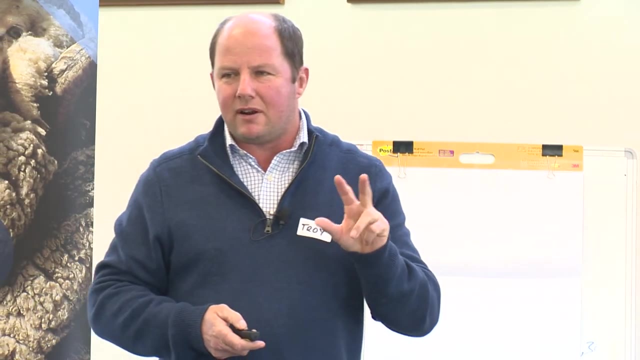 just different rice crops and how much revenue they generated per megalitre. so that's. we all know that there's different years as well. yeah, so there's really only two years that rice was grown. yeah, it is what's across the bottom scale, the number of rice crops. so 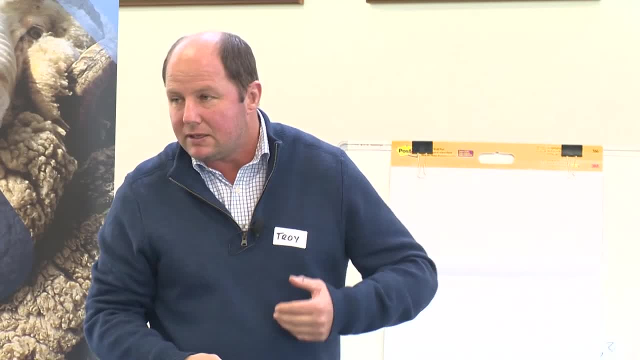 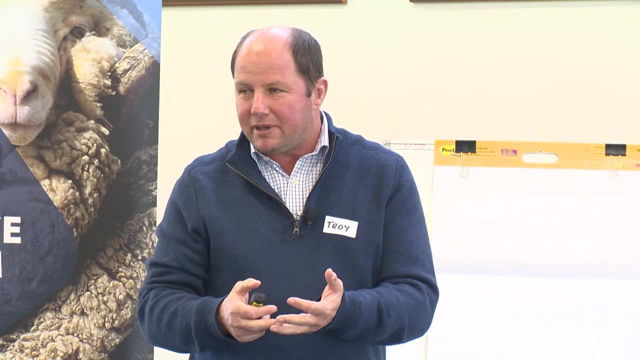 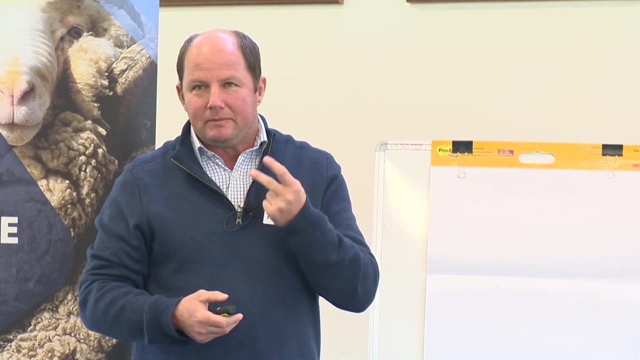 there's 25 rice crops within that over that period of time. yeah, so some- obviously only probably four people grew two rice crops in that period and obviously 12 or might have been a bit more than that, but yeah, not everyone grew um two rice crops. um, yeah, so some people might have grown. 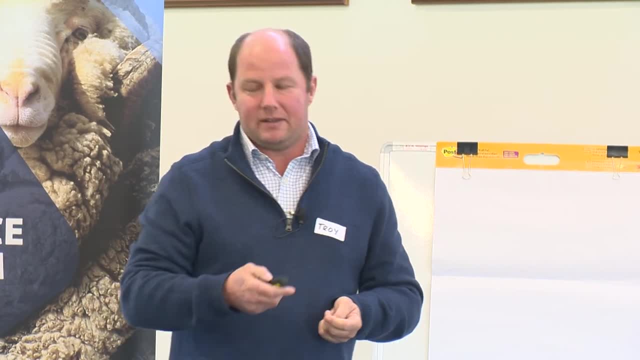 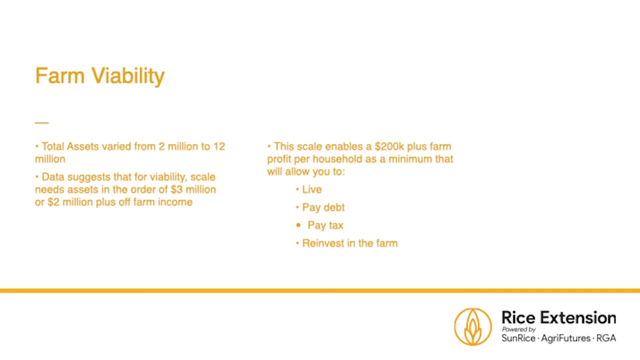 a crop every year and something might have a couple of years out. that's it. yeah, yeah, uh, farm viability. so they, yeah. what did we find? uh, total assets varied. amongst these is this group of farmers from 2 million to 12 million. data suggested for farm viability: you need, in order, about three million dollars. 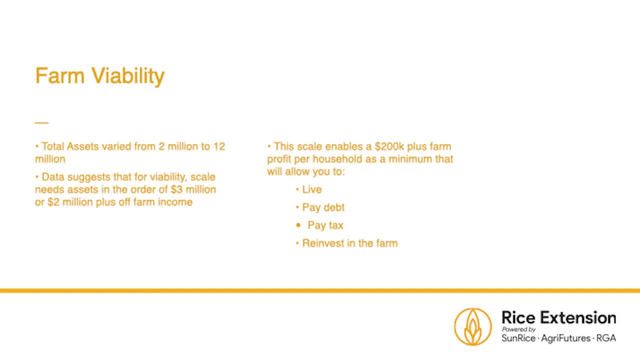 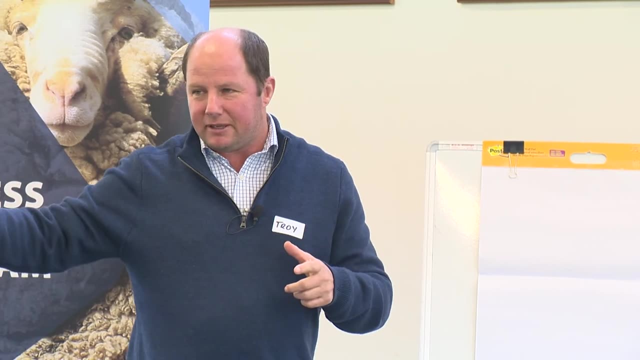 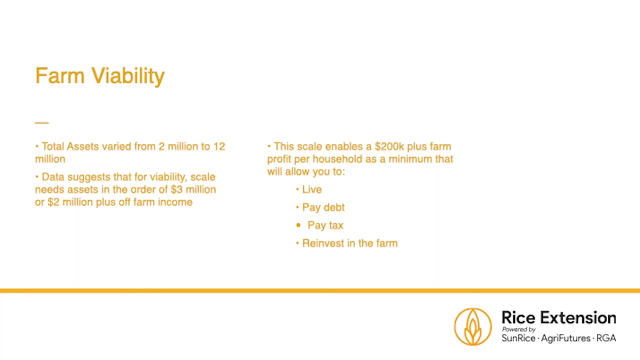 in assets per household, or you can have two million in assets per household, so remember that word per household. so if that's just mum and dad, but if you've got, you know, two kids on the farm as well, that's another two million each for them. that two million- that's the off-farm income- had to be regular and it had to be pretty substantial. 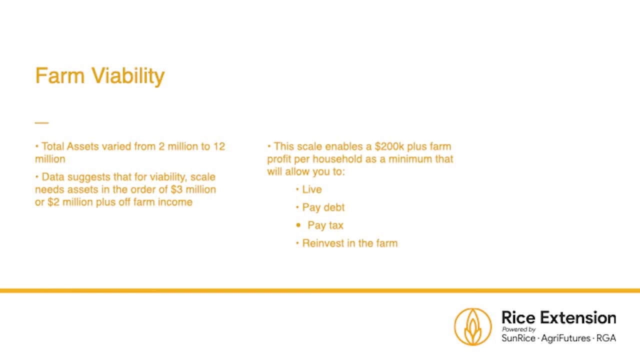 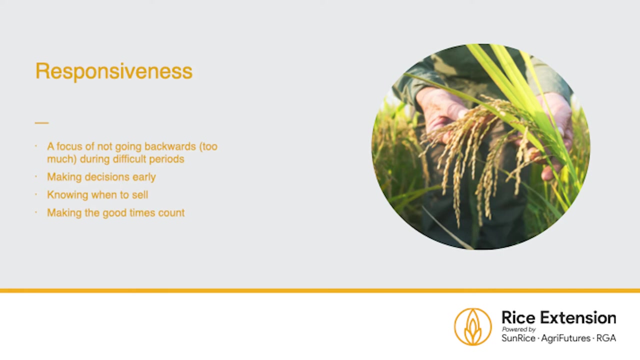 i guess. and that scale enables about 200 000 plus farm profit per household, which allows you to live, pay debt, pay tax and reinvest in the farm. so responsiveness, i guess. what did the good people? how did the better farms respond? there's a focus on 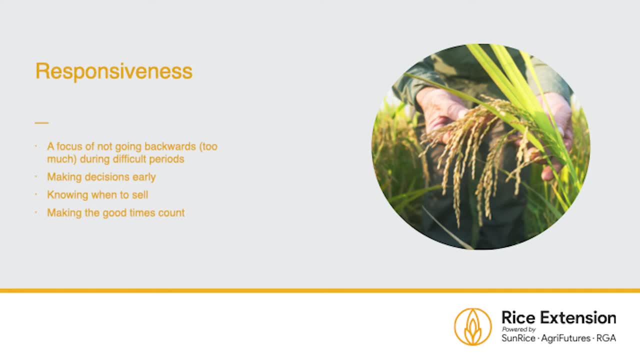 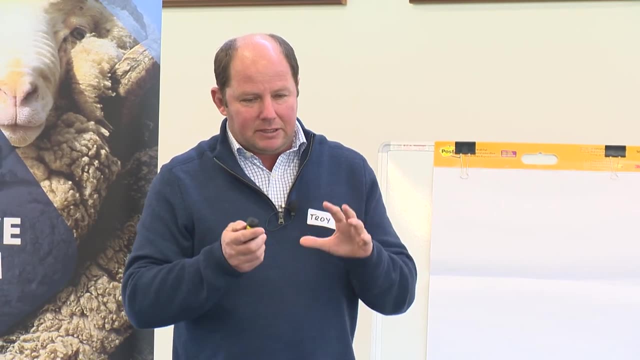 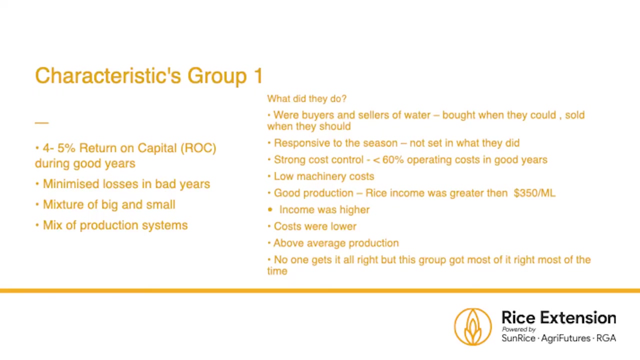 not going backwards in the hard years, making decisions early and knowing when to sell and making the good times count. so out of the 14, we sort of split them up into three different groups: those that perform really well, average and below average. the characteristics of the those that perform very well had four to: 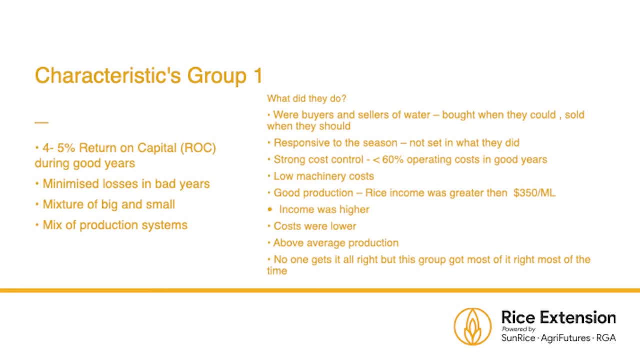 five percent return on capital in good years, minimized losses in bad years. once again, our mixture of big and small. so if you're asking that answer, it's not about how big or how small you're are mix of production systems. once again, there's no one answer. yeah, nobody, keep going. so what did? 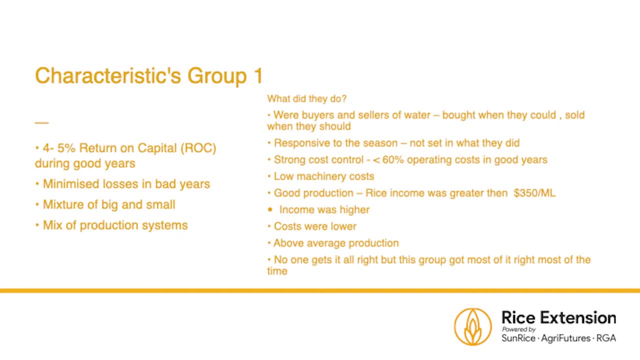 they do. well, this group weren't. they were buyers and sellers of water that really stood out. so they bought when they could and sold when they should. so certainly in years like this year they're buying a lot. if it's a, you know, zero percent allocation year, they're selling. 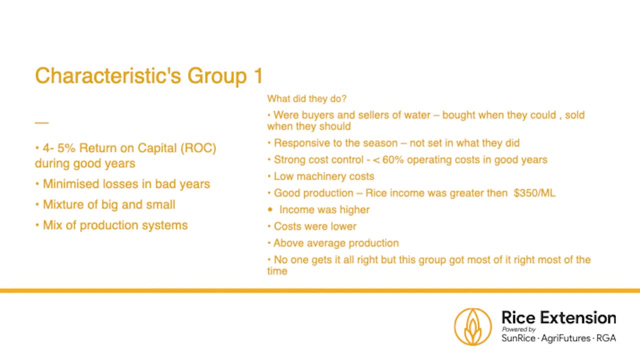 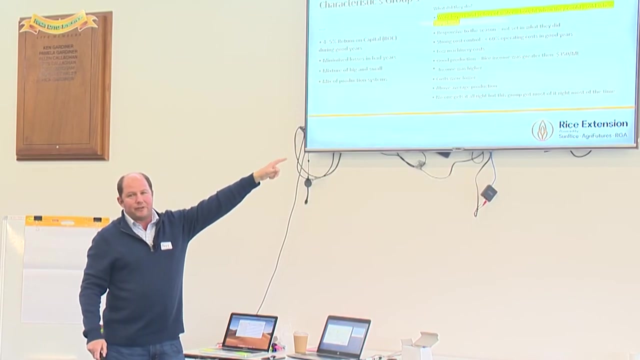 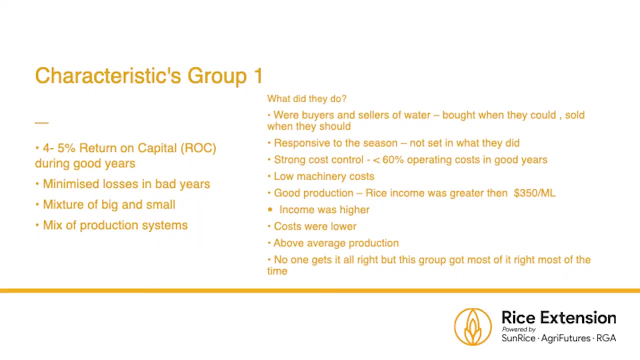 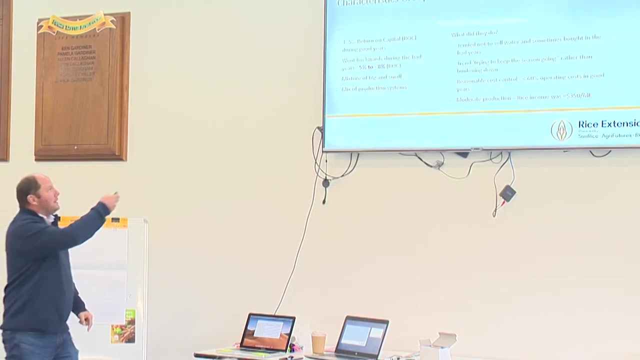 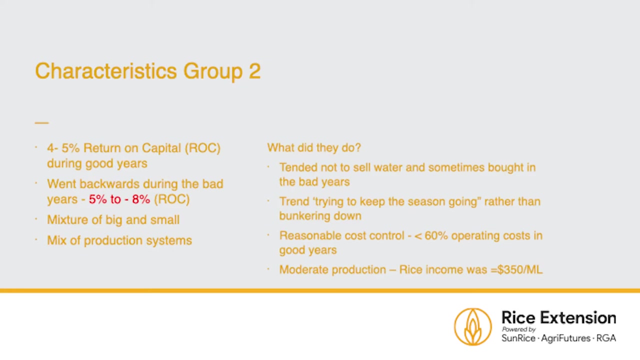 they respond to the season, not setting what they, what they do, very flexible in their planning. you can see that also with the our second group had. so they had a good return in the good years but they went backwards in the in the two drought years. on return on capital, I tended not to sell water and 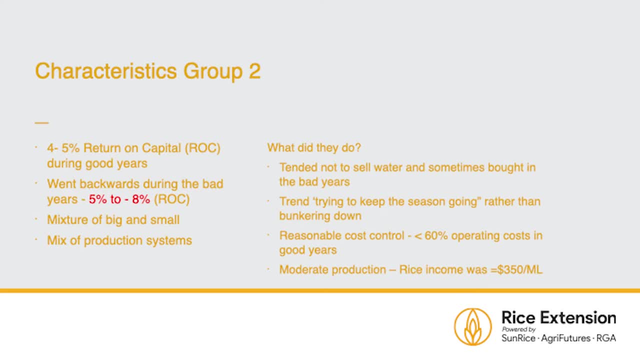 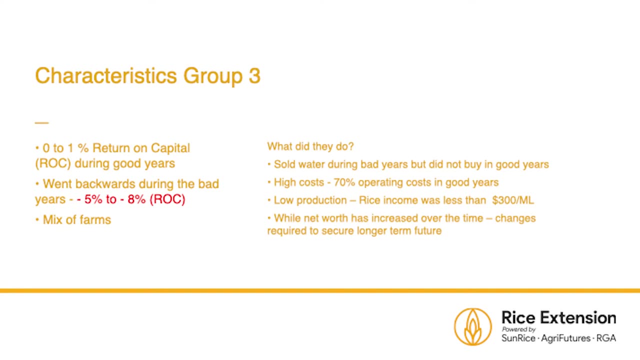 sometimes bought water and moderate rice production. so a couple of points. the third group, which shouldn't do that well. so I only had a zero to one percent return on capital in good years and went backwards in the bad years. once again, mix of farms. they sell water during the bad years but didn't capitalize when. 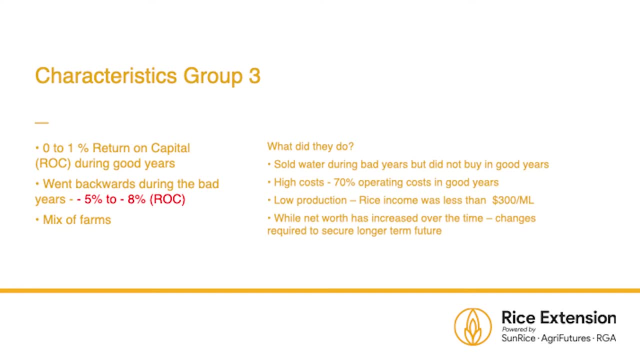 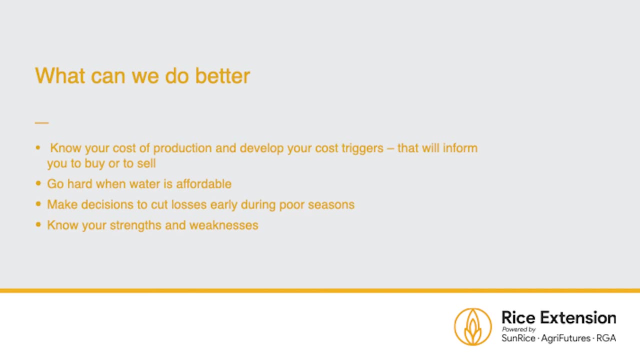 it's good when there's lot waters, plentiful. that was the main difference. and obviously, while their net worth increased over time, changes required. obviously, what can we do better? know your cost of production to develop your cost triggers. that's about that: buying and selling water. now your cost of. 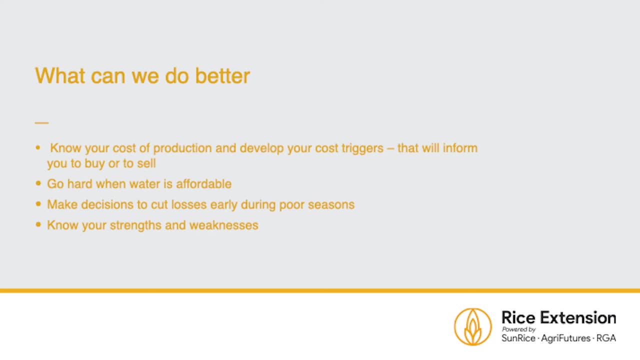 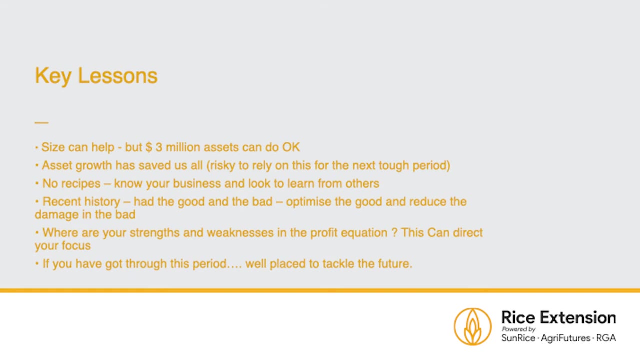 production. when you should buy and sell, go have and water is affordable. make decisions to cut losses early during poor seasons. know your strengths and weaknesses. size can help. as we said, asset growth has saved us all. there's no recipes. know your business, look to learn from others. so there is no one rule for all of us, whether you 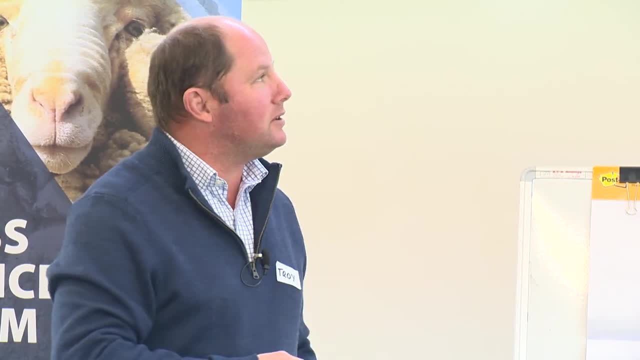 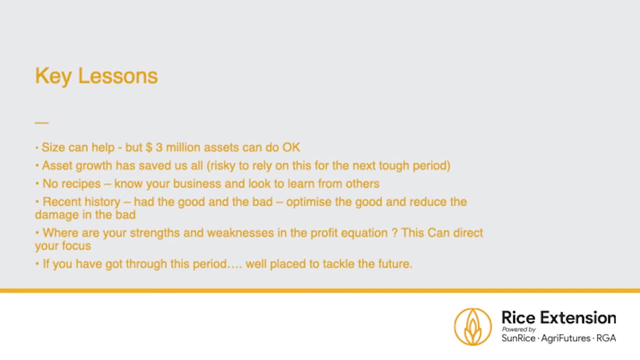 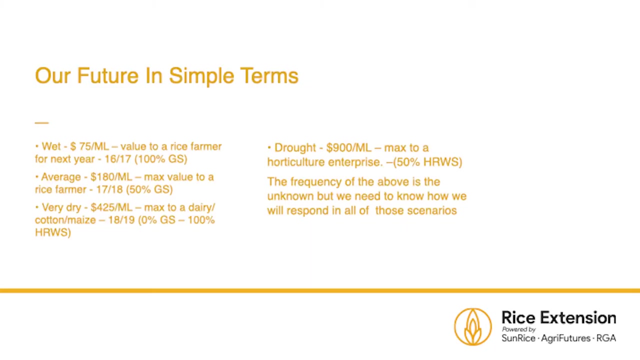 have lots of water, big farm, small farm, livestock or not, how much? if you got through this period, you're well placed to tackle the future in simple terms. in simple terms- and I presume you might touch on this too, Rob- if water, if it's a wet air and waters at 75 bucks, it's great value to the rice farmer. if it's. average like 17- 18. we had a lot of water in the past and now we've got a lot of 50 percent allocation. that it's 180 dollars, was the average water price and it's a max value and I'll show you that in a minute. that rice can pay very dry. 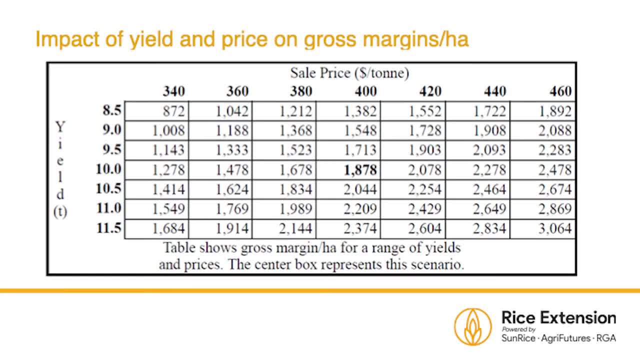 etc. so right, so this is where. so this is the gross margin of rice and I'll probably just go to this next one, which is per megalitre. so what we say, this is based on 13, using 13 Megs a hectare of water per year, and if you look at the 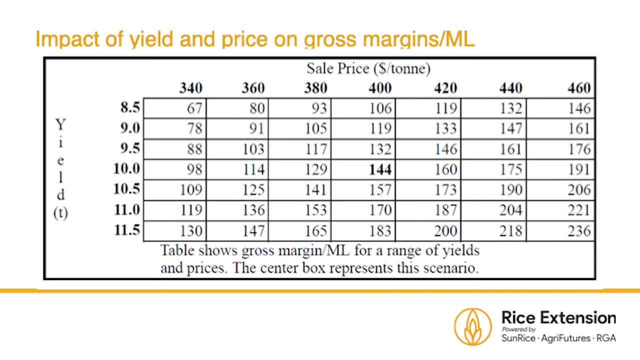 price of $1800, which is about 14% in the US. we have a big-up value in Australia. there, and you know, purchase water. so what we can see from this matrix is to where we said we topped out at. the 187 is 11 ton and for $20 a ton. so so down. 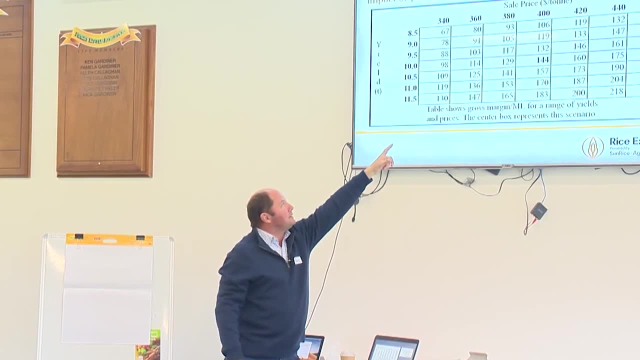 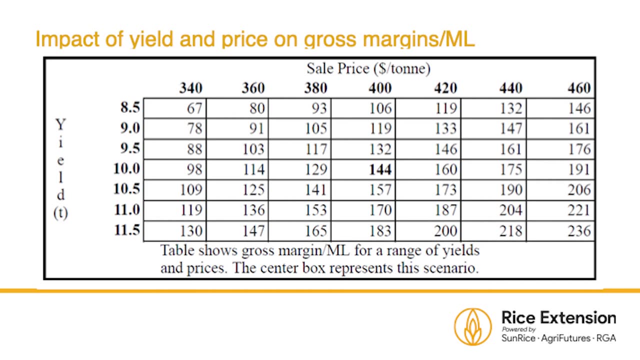 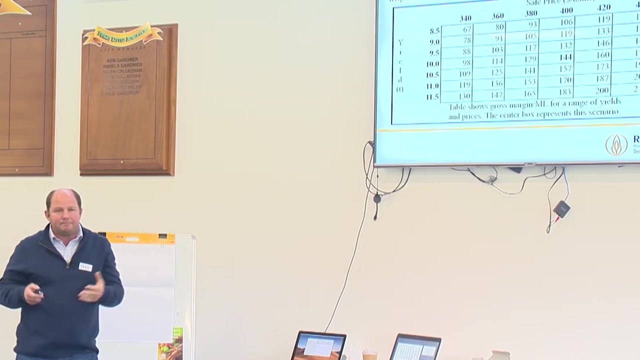 on our the column. here's our yield and across there is the price of rice. so 13 megs at the at $400 price, the returns coming $144 per megalitre. so that's at full contract prices. so that's where you say, obviously if you do it yourself, if 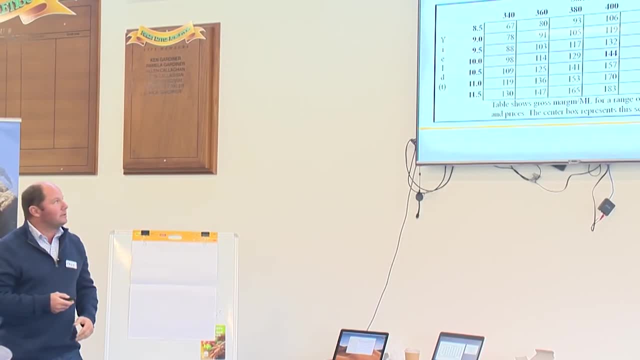 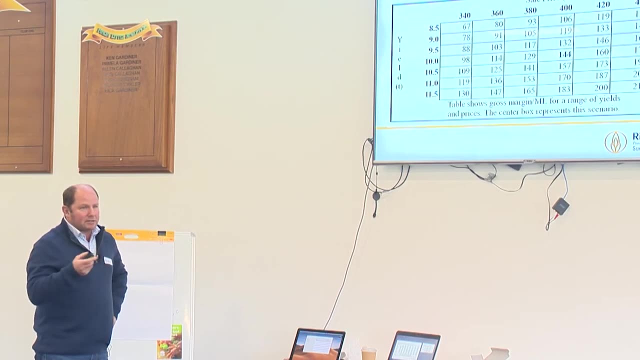 your harvest and all that. you're going to have reduced costs, so your gross margin will go up a little bit. to give you an indication- and I actually did these in March when we were originally going to do the this workshop, and it's funny what has changed so since. 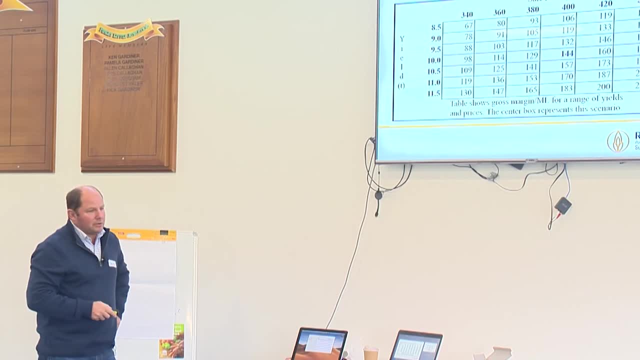 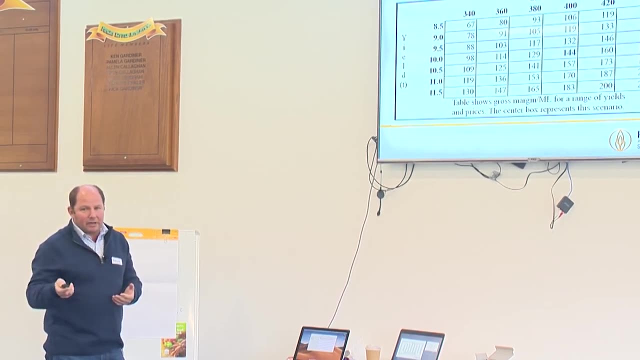 then I use 10 as an average yield. that was on the back of receipt, which is about five year average. for here we've now got a new variety called via 71. I just looked at the data this morning. it's averaging about 12 ton for the. 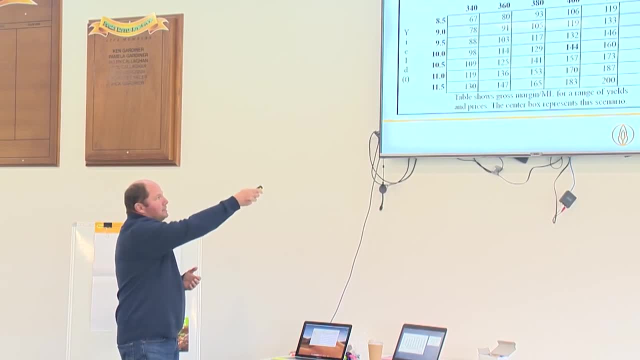 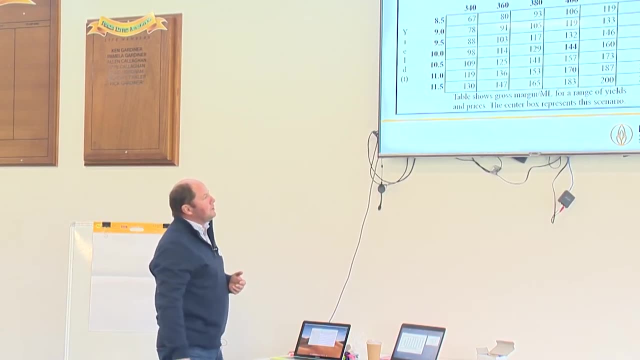 whole valley. so so it's a big step change. so that's where we can. we'll get a higher return per megalitre. we'll get down past, you know, $200 a meg, but generally it's at $100 per megalitre. so that's where we can. we'll get a higher return per megalitre. we'll get down past, you know, $200 a meg, but generally it's that one. 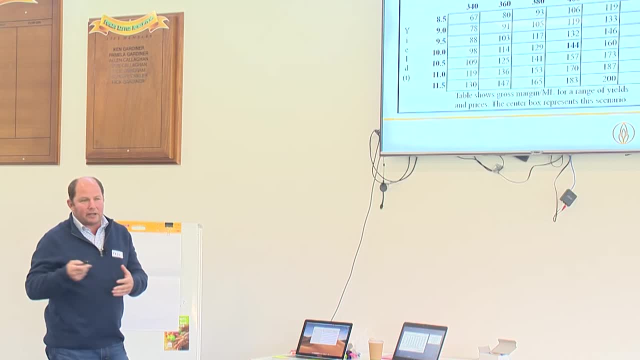 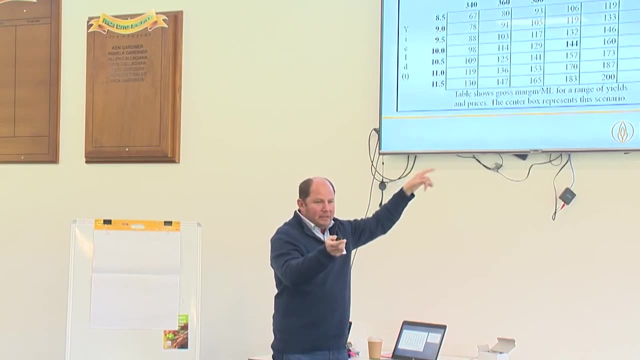 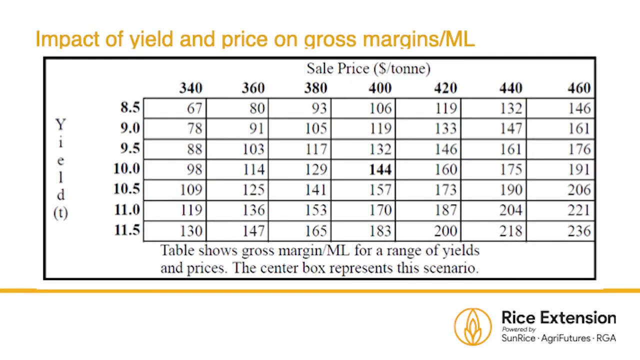 83 is about the max out, so I wouldn't be relying on that 12 ton. year in, year out, we've had an exceptional year, but that's where- yeah, and so this is done. yep, yeah, 420, and obviously that helps as we go. yeah, so the the price guidance for this. 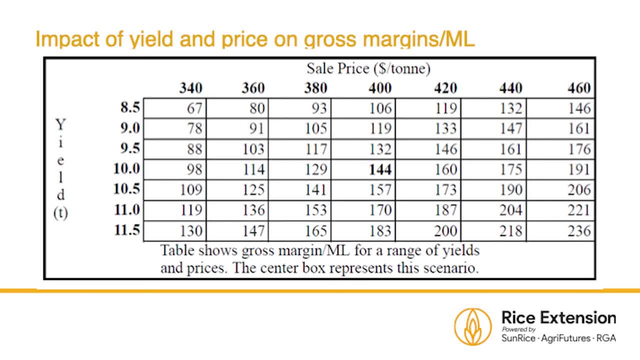 year's crops 390 to 440, I think, or 430 but round that 440. so yeah, but it's a good start. obviously, if you get less yield you're not doing as good. we all know that. we're not saying that's what we can afford to pay for. we're saying that if 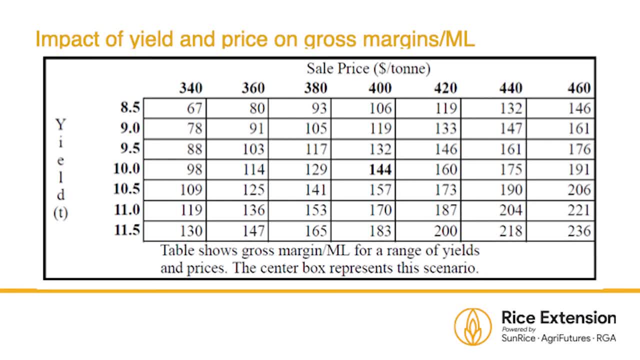 we grow a crop with water, that's the return. like for every megalitre we put into it, that's what we'll get. yep, so then if you're going into the market to buy water, you've got to factor that in and see whether you know if you're happy. so that's what i've done here, dave. so 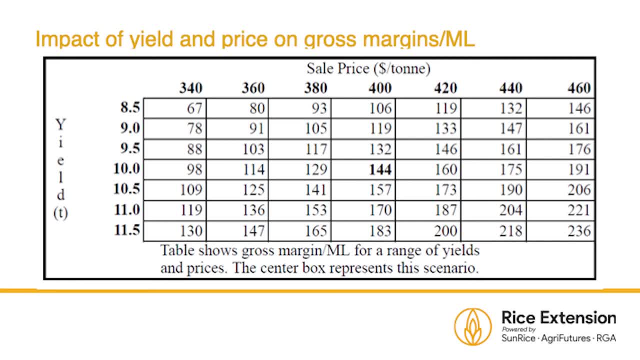 i've bought water for fifty dollars. my return is 132 megs. so if i can get it cheaper, my return obviously when you buy it for 20 and rob's going to tell us how much we're going to pay next year. so we get it for 20 bucks and i do 10 ton, which is 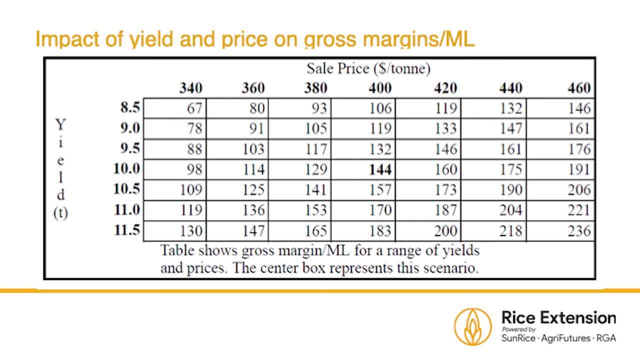 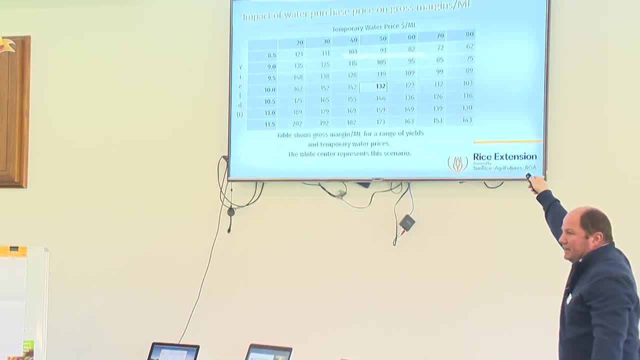 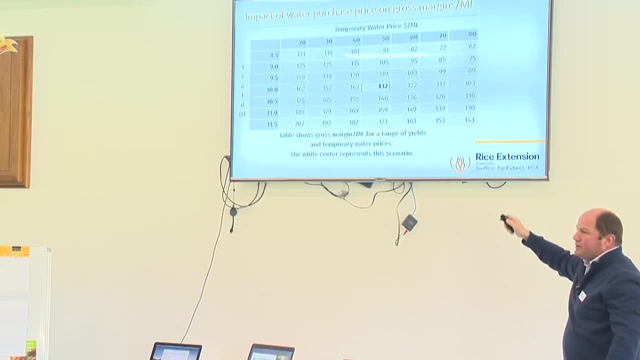 that five year average for a receipt 162.. so i've paid for me water plus i get 100. likewise, if i come up and if i pay 80 dollars i'm going to get 103 at that 10 ton. but if i grow 71 and it goes well, i'm up 130, 143. so that's just showing. 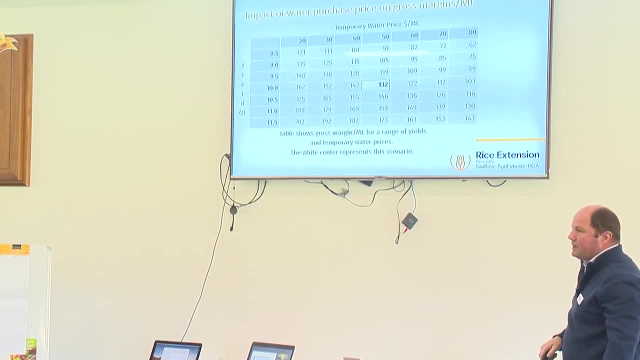 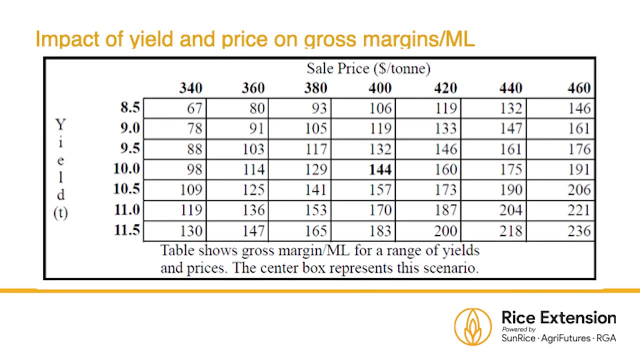 the impact on the price of temporary water that we pay. but just going back to here, so remember. so in the analysis we come up with that figure of 185. so this is just a gross margin and it really lines up with that figure. so we're all on the same page. 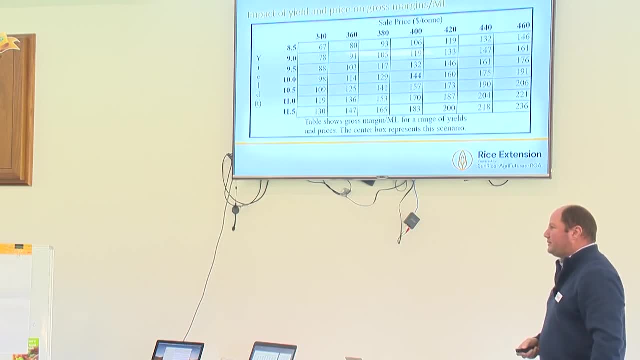 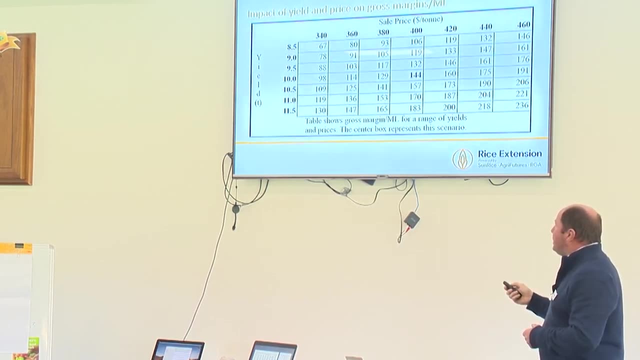 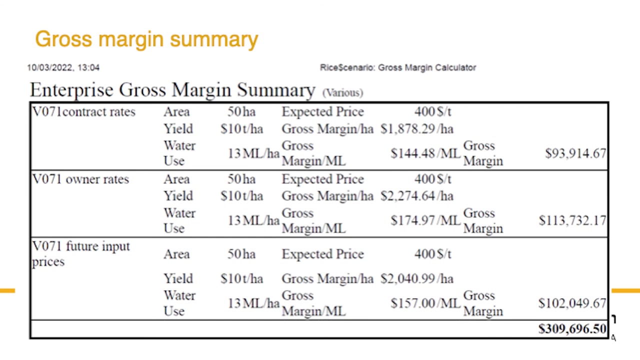 i guess one's theoretical. well, it wasn't theoretical, it was taking in account of that data and this just really proves it. so, uh, any questions? so this is also just a summary of how our gross margins can change. so, as i said, the first one is using va71 full con contract rates. 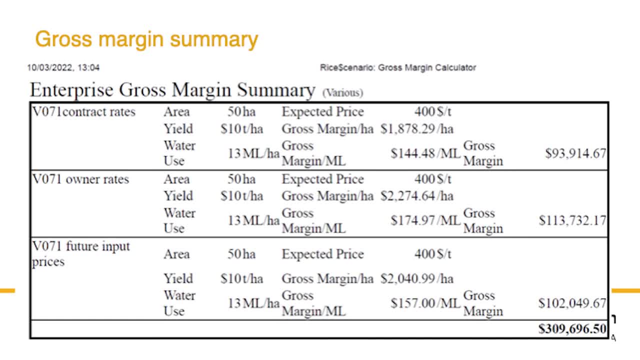 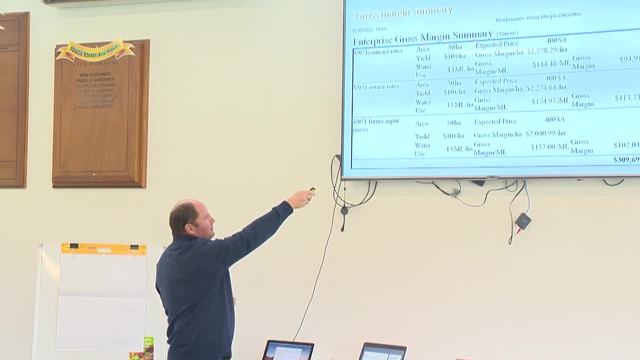 the next one's owner rates. so as i do, that is, i have the cost for harvesting cartage and just your operations, so you can get a higher gross margin of 174.. likewise, as i said, this is using 13 megs. if we use this year, we use less water. 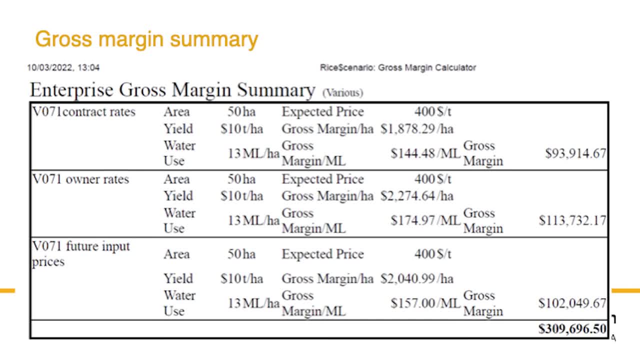 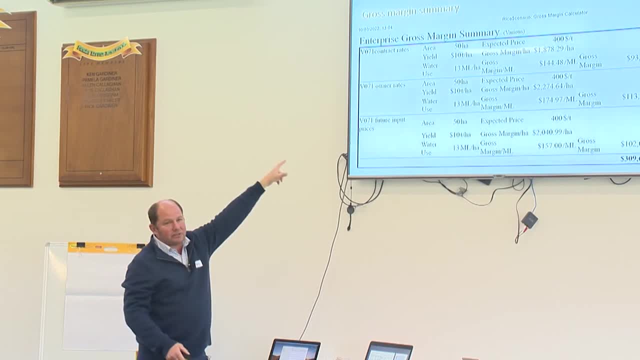 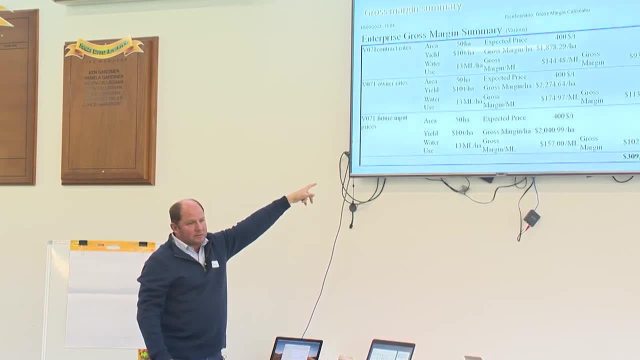 so if we use 11 megs, that gross margin would go up to 200 a meg, uh, and then va71 with future input prices. so the first one that was using euro at fifteen hundred dollars, map, because that's how much it was in march. this next one is using a thousand dollars for them, and